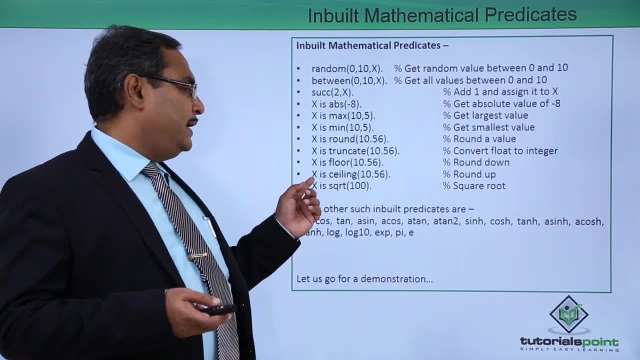 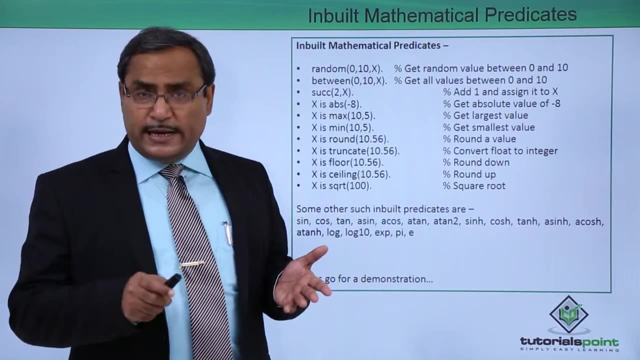 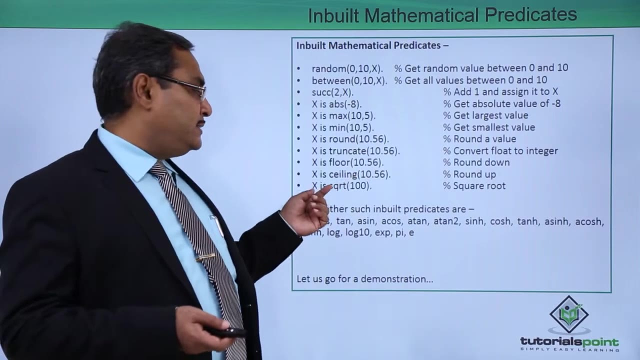 So the value will be 10 in that case. So 10 will be assigned to x. x is ceiling 10, point 5, 6.. What is the ceiling? Ceiling means the smallest integer larger than this number, So that will be 11.. So 11 will be assigned to x. in this case, x is square root of 100.. 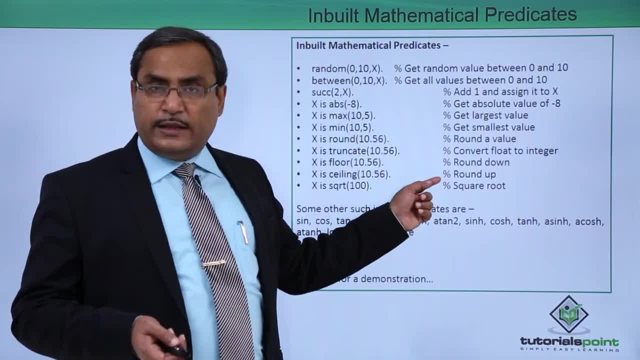 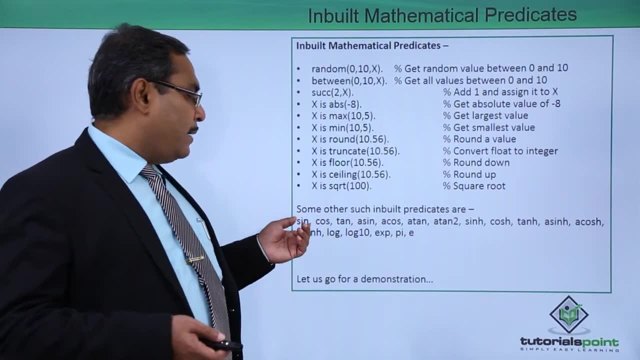 So 10 will be assigned to x. So we have written everything in the comment. So this percentage symbol indicates we are writing a comment for that. Now we are having so many other mathematical functions and predicates. You can use them. 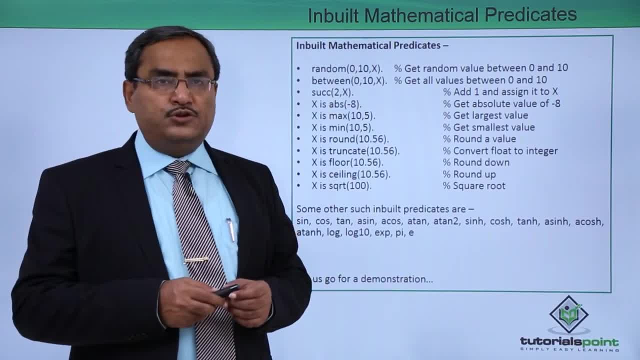 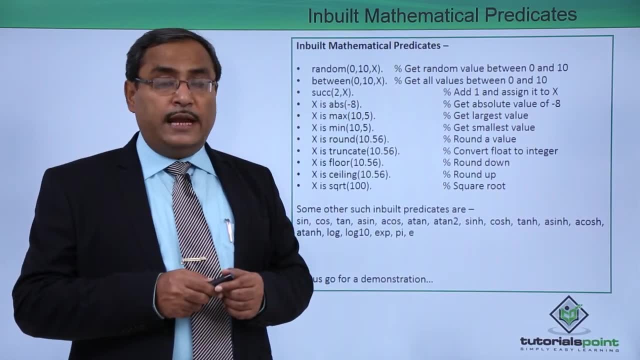 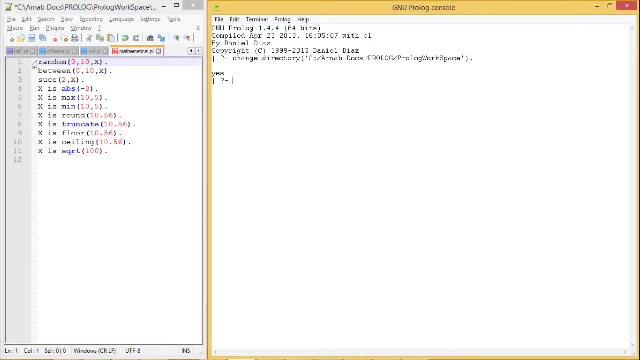 in your prolog code. So let us go for one demonstration where we shall show you these mathematical predicates- or you can call it as mathematical functions- how to use them in our prolog code. So here is the demonstration for you. We are going to execute these inbuilt. 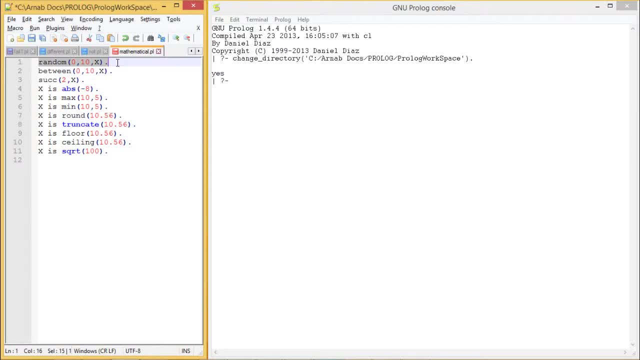 predicates. that is random, between successor, absolute max min and so on. So let me execute one by one. let me show you that how they are producing their respective outputs. so here you see. this random predicate is generating numbers ranging from 0 to 10. 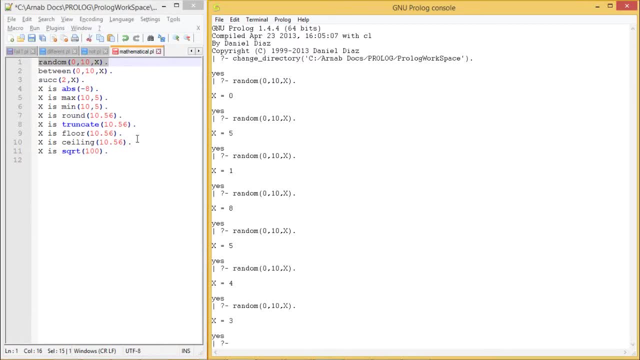 in a random order. so in this way you are getting this idea. it is generating all numbers between 0 to 10. it will generate the next number. so if we make this one as 12, then it will generate 13. ABS will only consider the magnitude part of the number: sign part. 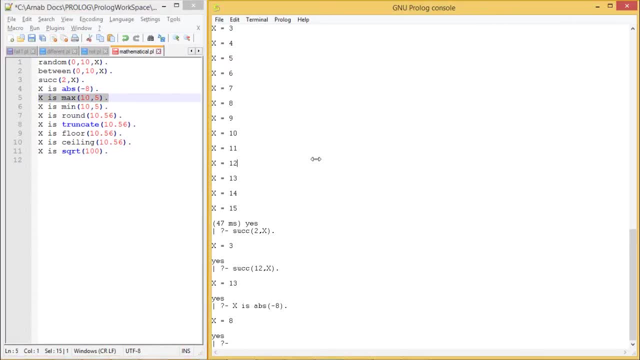 will be ignored. so max is there inbuilt, which will give you the maximum of two numbers. similarly, for minimum, it will give you the minimum of two numbers. round is here. so if you make this one as 10.156, then also it will give you 10. 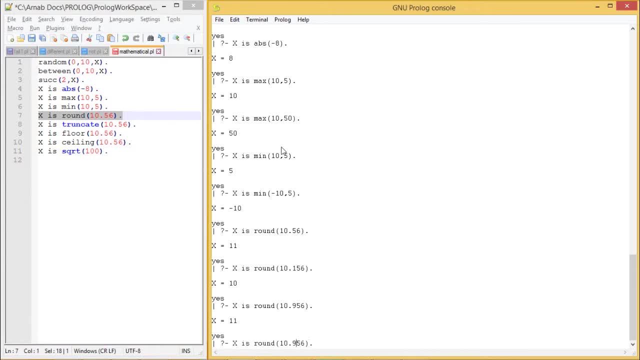 then it will give you 11. if you put here 4, it will give you 10. if you put here 5, it will give you 11. truncate 플레임. so it will just eliminate the fractional part. it will remain with the integer.